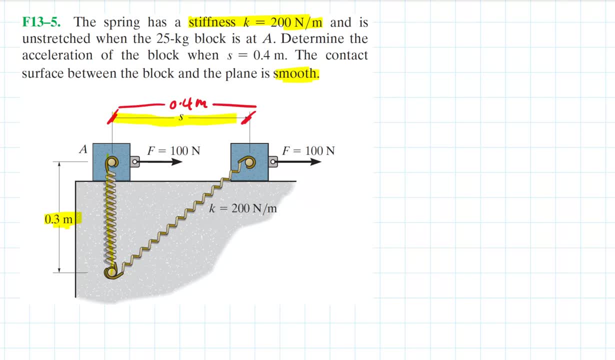 Okay, Another word right here. So, and this can form a right triangle And this is the stretched spring, So we can think of this as a triangle. This is 0.3.. This is 0.4.. When you take the square root of 0.4,, add it to the square root of 0.3.. 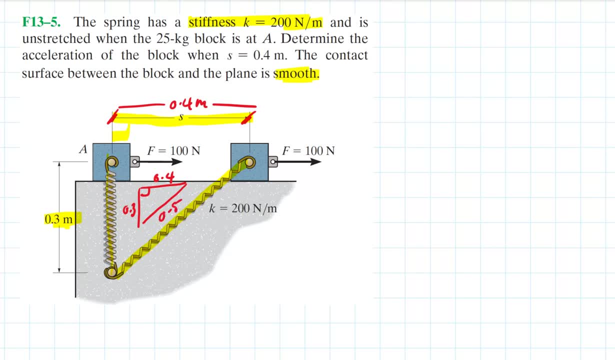 And take the square root, it will give you 0.5.. So that tells us that the distance from here to here is 0.5.. So how much did the spring stretch? So originally it's at? we said what? 0.3, right. 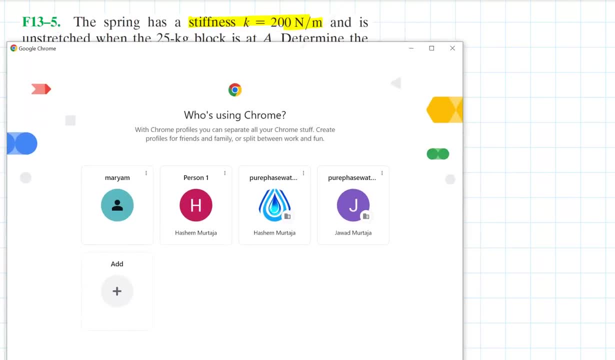 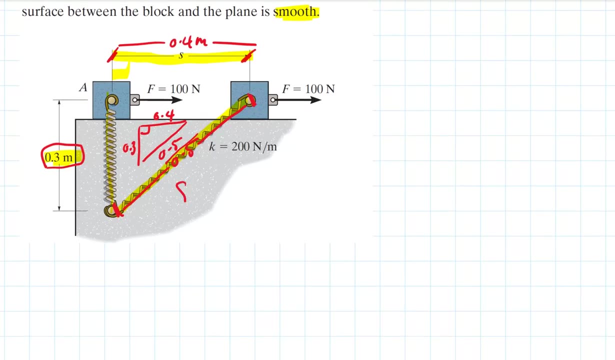 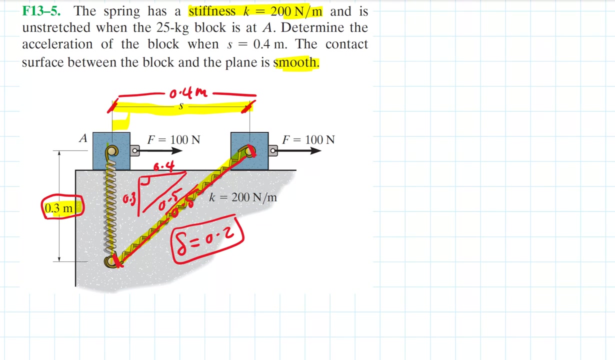 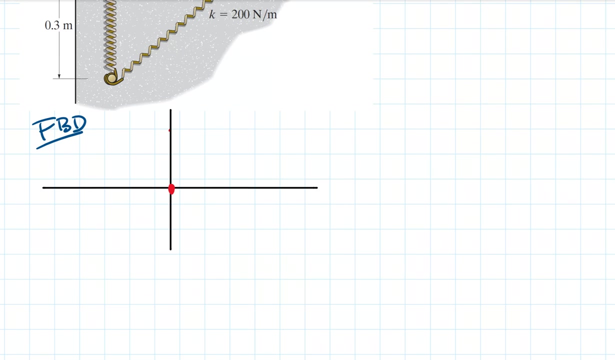 And then stretched, and the new and the new distance is 0.5.. So the difference between 0.5 and 0.3. So the displacement, is 0.2.. All right, So now we will draw the free body diagram of the 25 kilogram block. 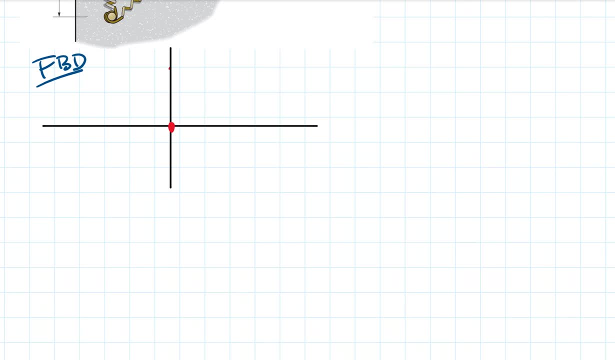 It's 25, right, Yes, 25.. Okay, So the first force we have in here is our 100 Newton force, And here we have the force due to the spring, And we can break this into vertical component and horizontal component. 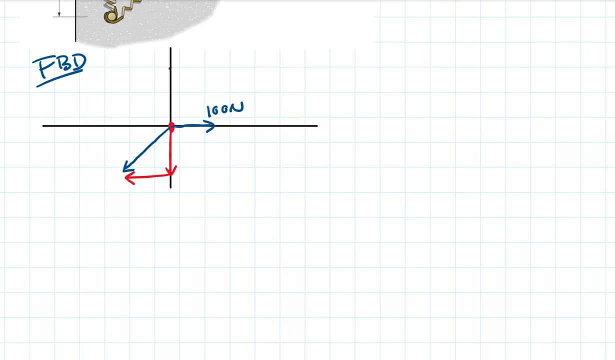 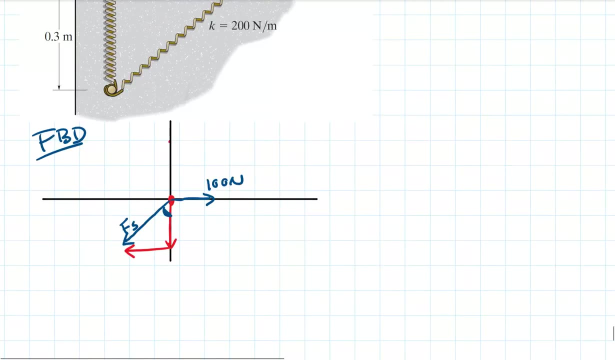 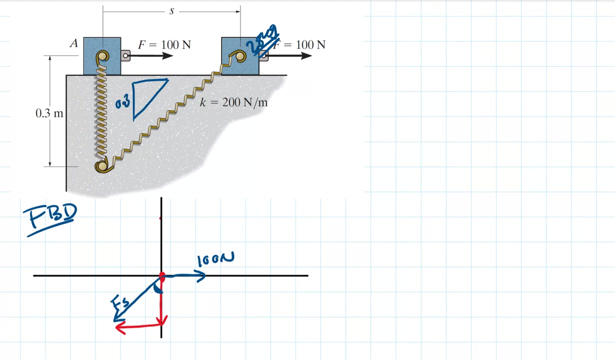 And we can. we say: this is the force of the spring And this is, and we can use this angle right here. So here we said that we have this triangle like this: Remember: 0.3, 0.4, 0.5.. 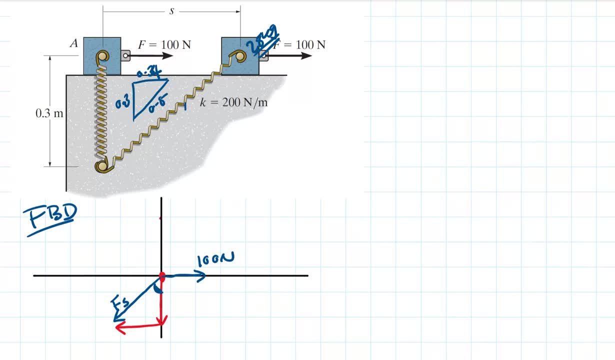 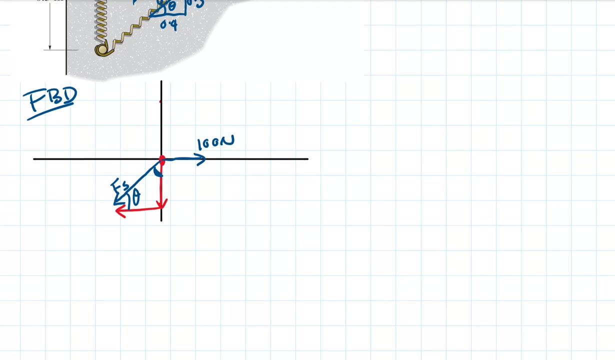 So, if we flip this right here, 0.4, 0.3,, 0.5.. And this will be our angle theta. Okay, So, so what? we will use this angle theta, which is this angle theta right here. 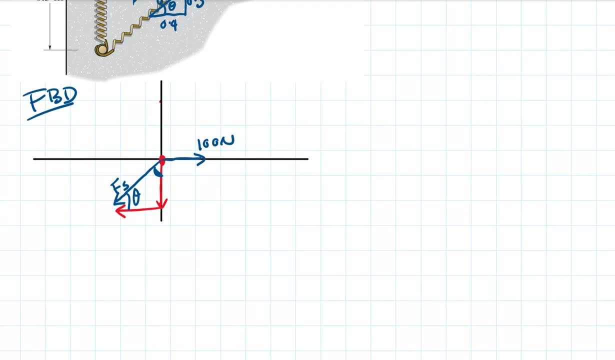 All right, And here obviously we have the mass due to gravity and we have the normal. But here we will not add the forces in the Y direction, because there is no movement in the Y direction And there is no friction, because here we're told that we have a smooth circle. 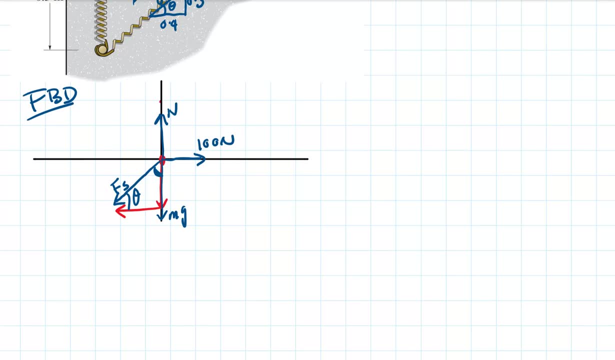 We have a smooth surface because friction is related to the norm, to the normal force. So here we will say that the sum of the forces where it this thing will move to the left, The sum of the forces in the X direction equal to mass times acceleration in the X direction. 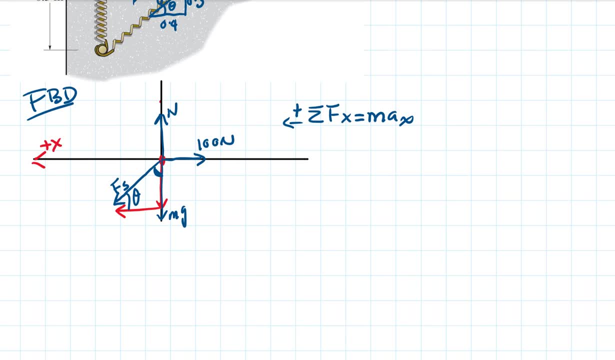 So let's say so. this will be your positive X axis, This will be your positive Y axis. No, sorry, This is wrong. It will be different. Positive X, All right. So, right here to the right, we have our 100 Newton minus the horizontal component, which 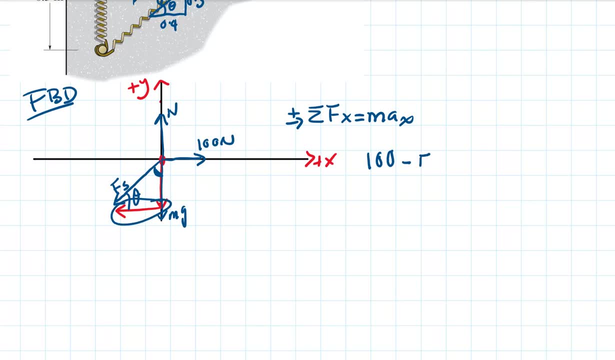 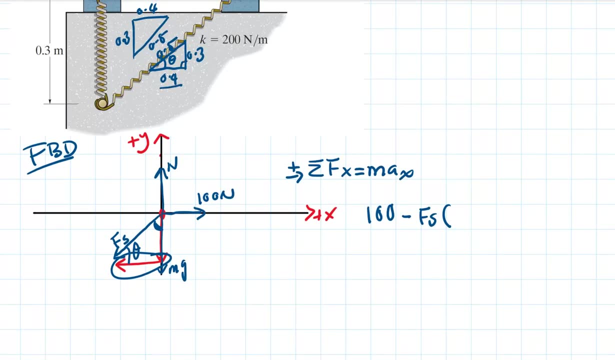 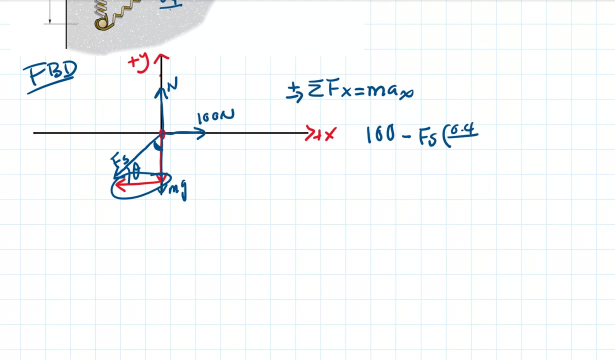 is this which is force of the spring times. since this is adjacent, So it will be 0.4, and the cosine is adjacent over hypotenuse, So 0.4 over 0.5.. 0.4 over 0.5.. 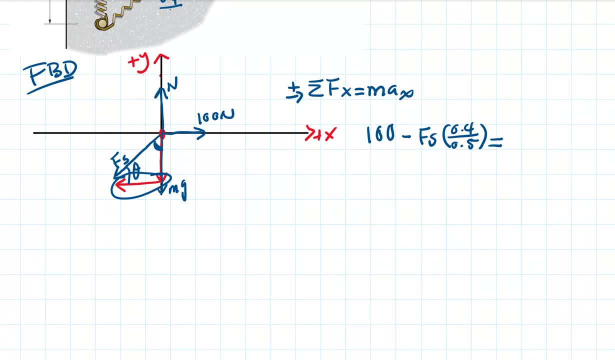 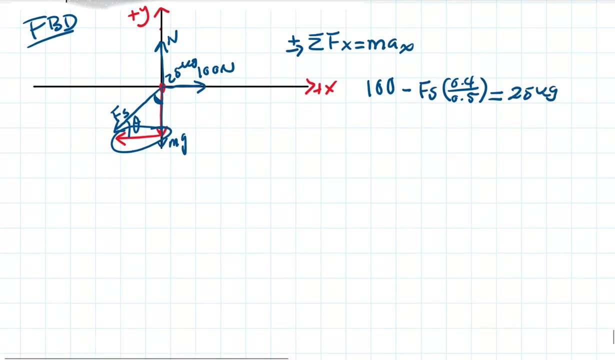 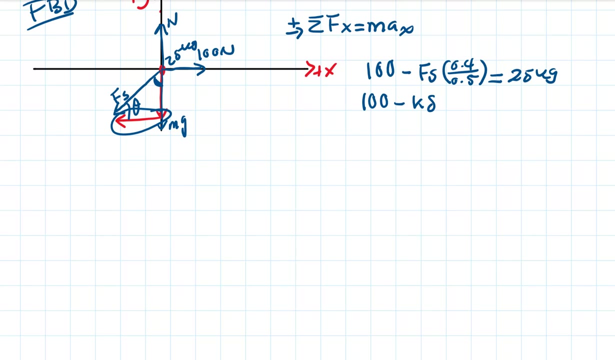 Equal to The mass is 25 kilogram, 25 kilogram. So you can say that 100 minus the force of the spring is what is the spring. constant times: the how much the spring got stretched or compressed Times 0.4 over 0.5.. 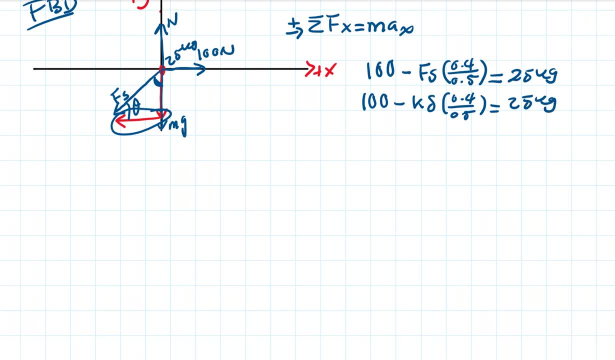 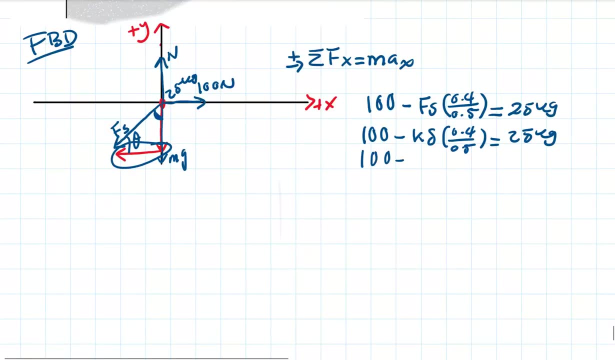 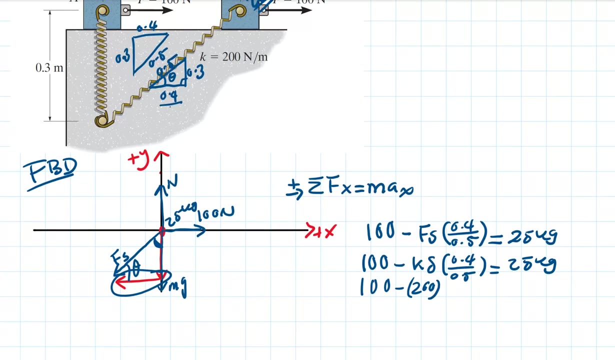 Equal to 25 kilogram, So that will be 100 minus K. We said it's 200.. The amount that's, that's being stretched. We found it to be point of the difference between 0.5 and 0.3, which is 0.2. 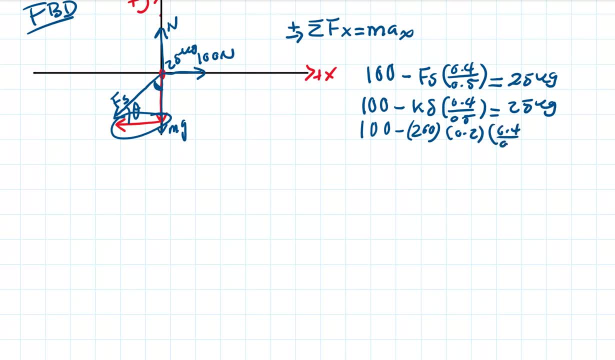 Times 0.4 over 0.5.. Equal to 25 times acceleration The X direction. So that will be what 100.. Let's plug this into our calculator: It will be 200 times 0.2.. 40 times 0.4 divided by 0.5 will give us 32.. 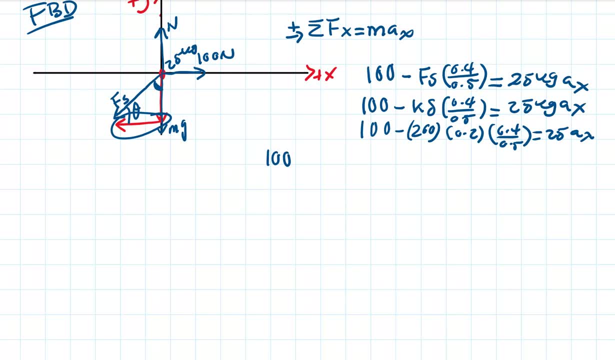 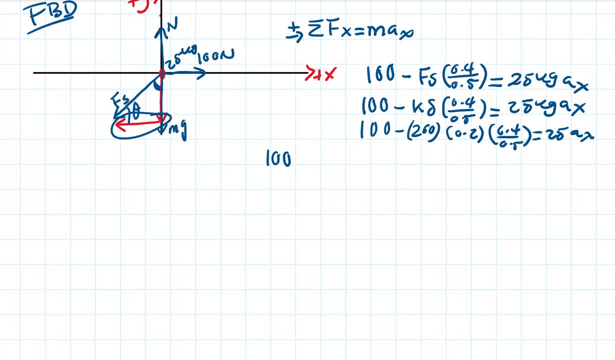 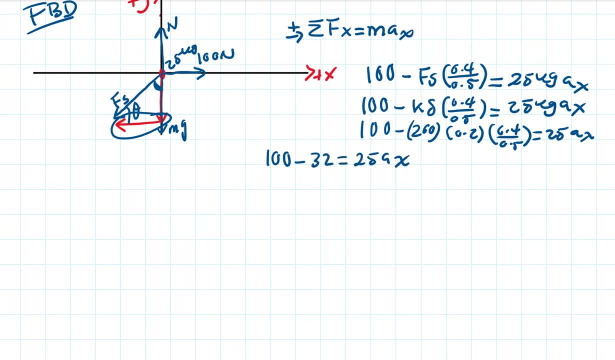 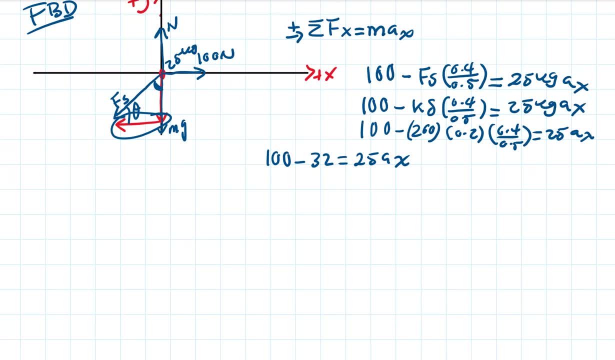 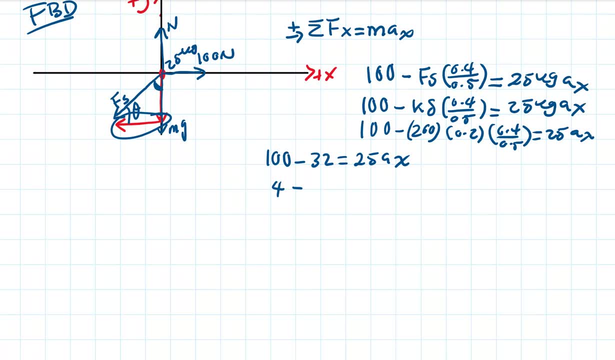 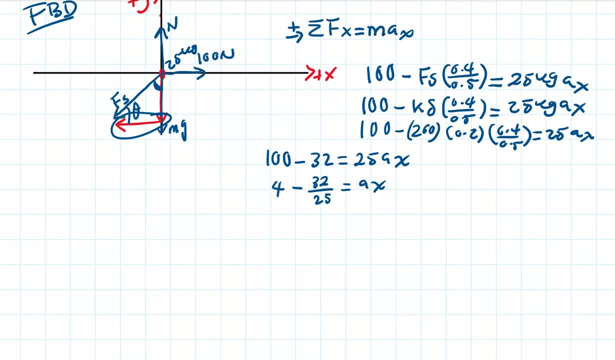 0.3.. 0.3.. 4 minus 32 divided by 25, and that will give us that the acceleration in the X direction will be 2.72 meter over second squared. so that will be our answer. and here a quick recall. any problem that you have relating to kinetics, it's always a. 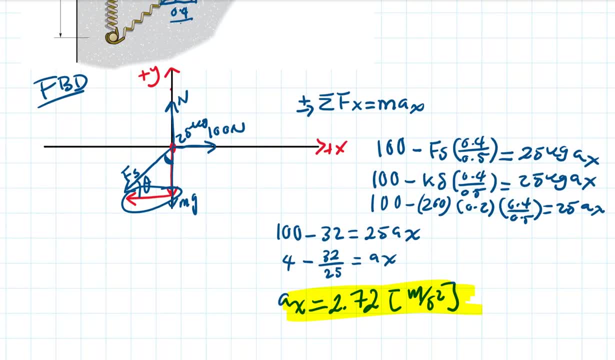 very, very good idea to make things clear for you is to always draw your free body diagram and spit and spin and make sure that you understand and you write down what is given. write a sketch what you need to find. draw your free body damn diagram properly. if you do that, you can solve your problems. no, no issue.